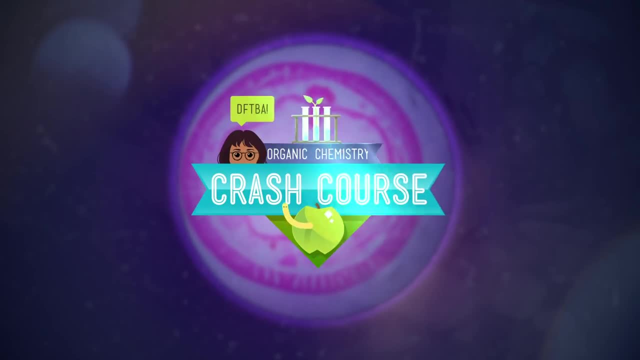 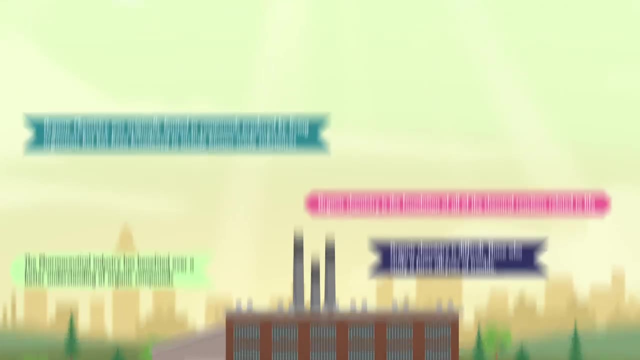 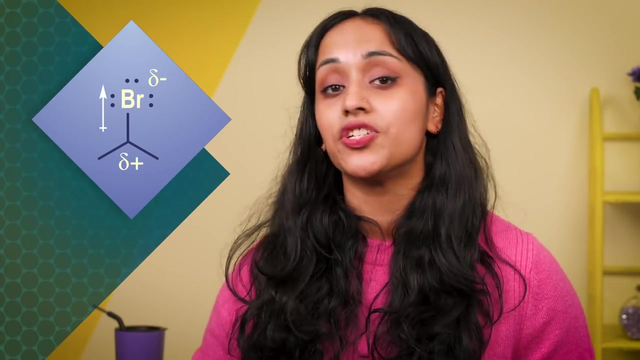 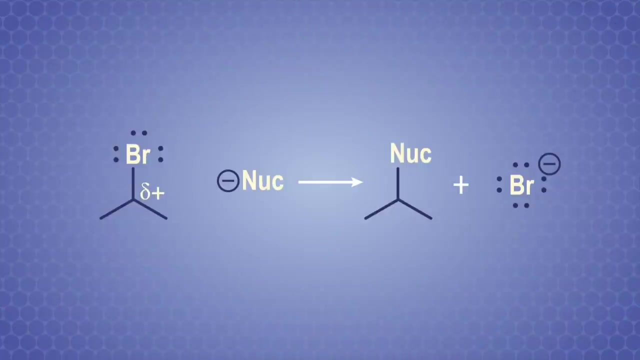 but may also have a dark side. INTRO: By this point we've mostly seen carbon bonded to more electronegative elements such as oxygen or halogens that draw shared electrons towards themselves. This gives the carbon a partially positive charge. 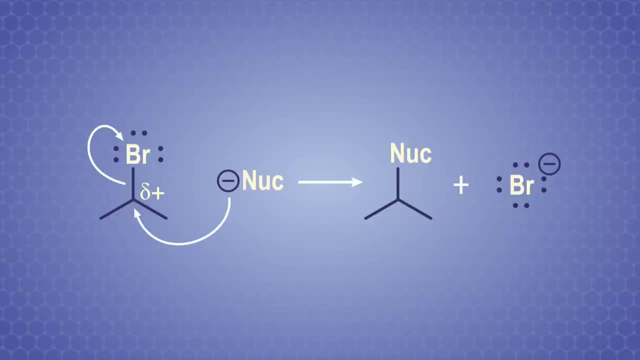 so it's susceptible to attack from nucleophiles, for example in substitution reactions. But metals are more electropositive than carbon, So in organometallic compounds the carbon in the carbon-metal bond pulls on those shared electrons more and ends up with a partially negative charge. 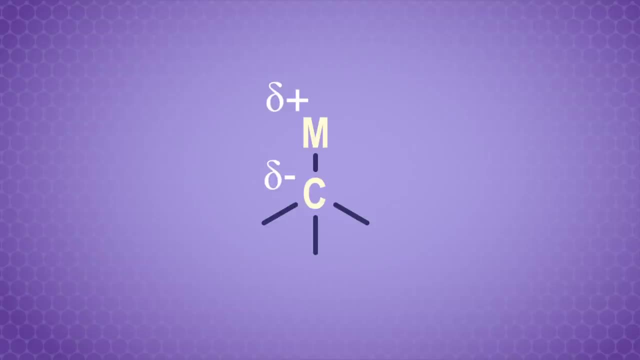 In other words, the carbon can become nucleophilic. In fact, we often end up with a compound with significant ionic character. The metal has a positive charge, while the carbon has a lone pair and a negative charge. a carbanion. 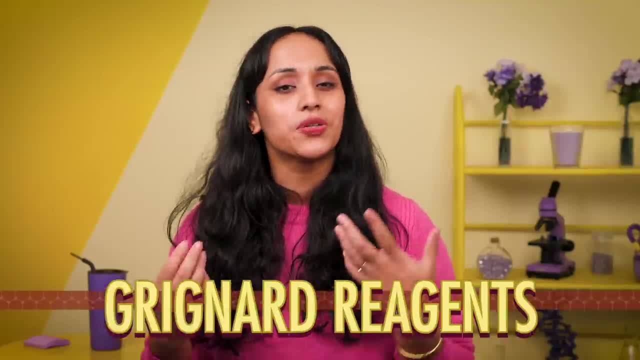 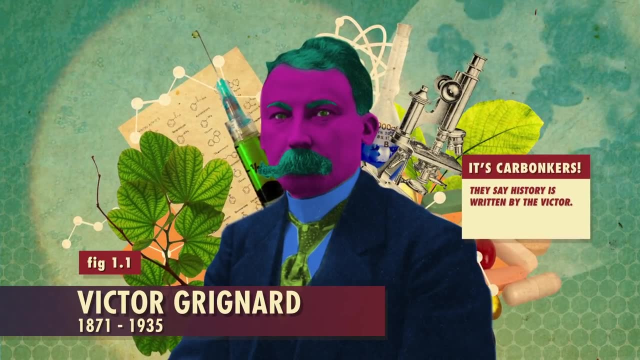 One of the most important groups of organometallic compounds is the Grignard reagents, which contain magnesium-carbon bonds. They're named after the French chemist Baudrillard, who said after the French chemist Victor Grignard, who won a Nobel Prize for his work in 1912. 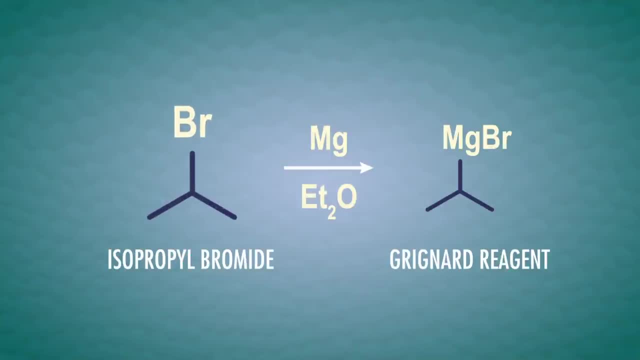 Grignard reagents sound quite simple to make. You add some haloalkanes, say isopropyl bromide to magnesium, in a flask containing ether And voila. But just one thing: keep water away from this concoction. 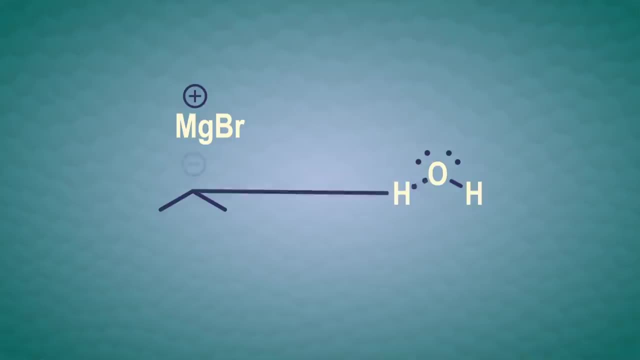 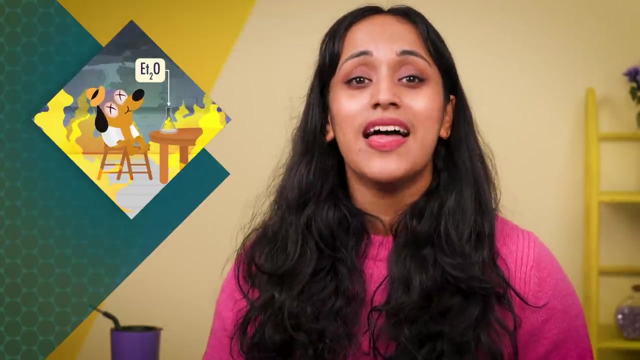 Because Grignard reagents react with acidic hydrogens to produce alkanes, which aren't the products we want. Oh, and another thing: be careful with the ether, because that's extremely flammable And since it's an anesthetic. 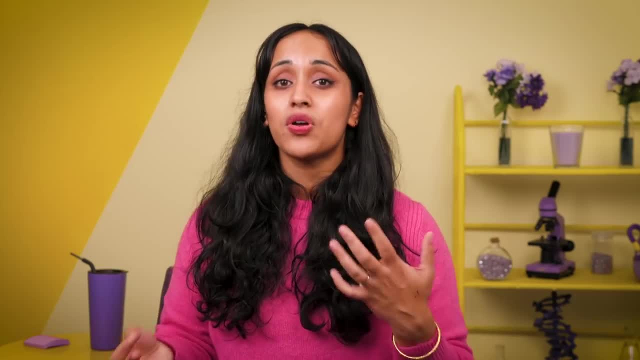 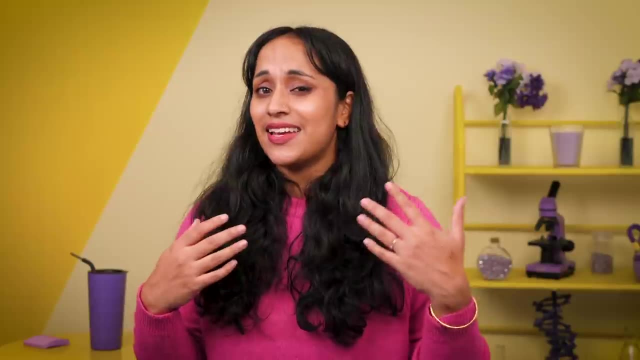 it may also knock you out while the lab is on fire. In fact, this whole mixture is described as pyrophoric, which means it reacts and burns in air. So yeah, it's… it's not that simple, Even though the dangers are totally different from tetraethyl lead. 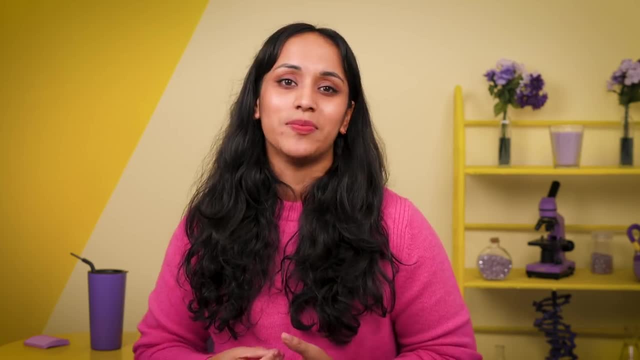 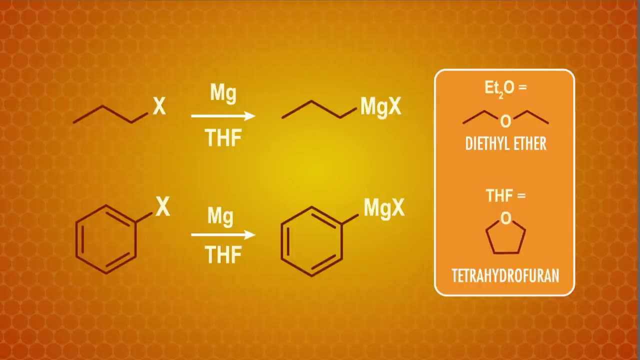 we have to be really careful about risk assessments with most organometallics. You can also make Grignard reagents by swapping the diethyl ether for a cyclic ether called THF or tetrahydrofurane. The lone pairs on the oxygen of THF. 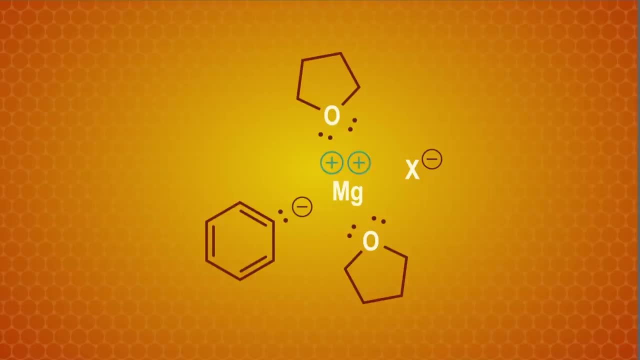 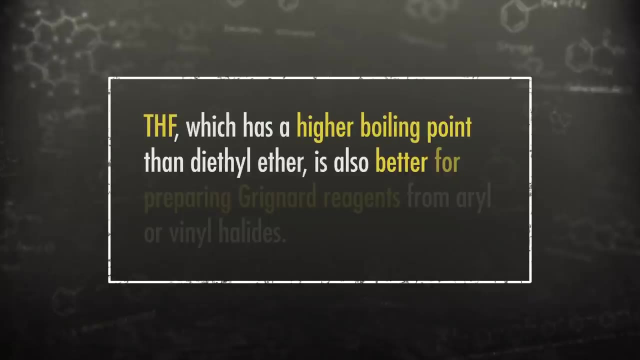 are more available to interact with a positively charged metal ion and this helps the Grignard reagent form. THF, which has a higher boiling point than diethyl ether, is also better for preparing Grignard reagents from aryl or vinyl halides. 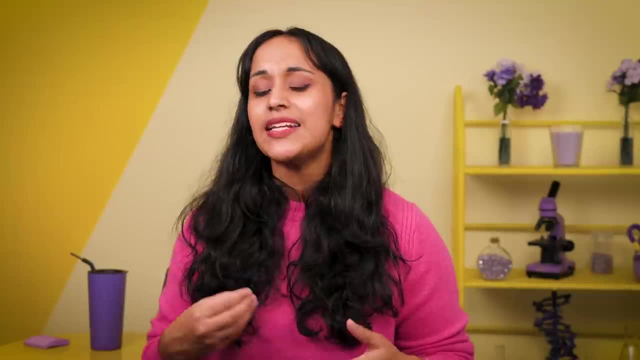 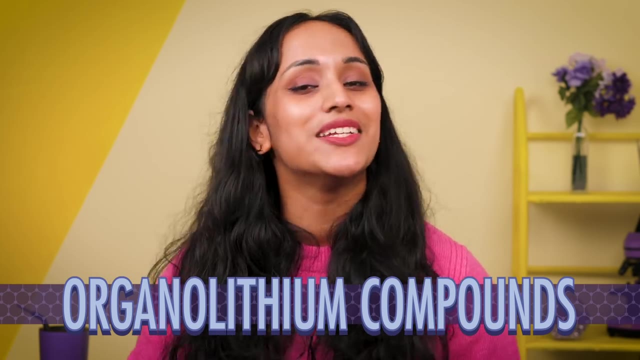 which react more slowly than alkyl halides and might need to be warmed up to get the reaction started. Other organometallics include organolithium compounds which, as you might have guessed from the name, contain lithium carbon bonds. They can be made in a similar way to Grignard reagents. 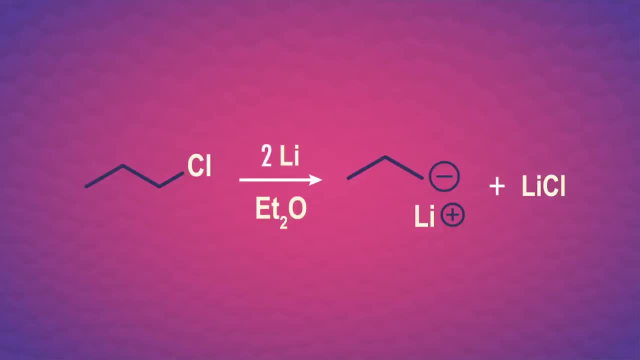 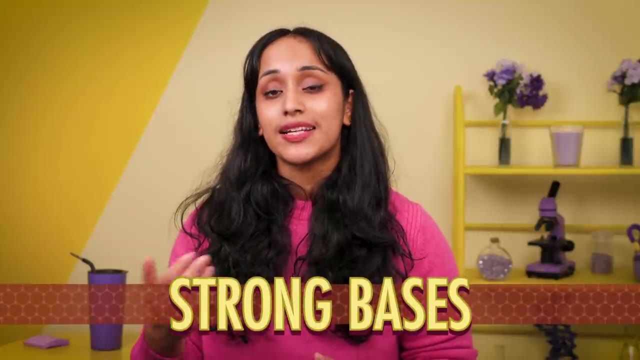 you add a halogen or a maloalkane to two molar equivalents of lithium metal, using ether as a solvent. Both Grignard reagents and organolithium compounds act as strong bases. They're proton acceptors and can rip hydrogen atoms off molecules. 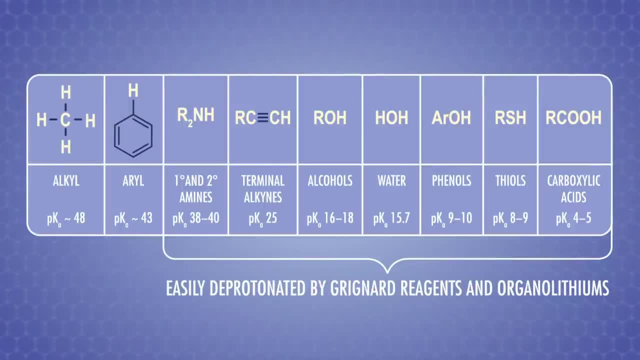 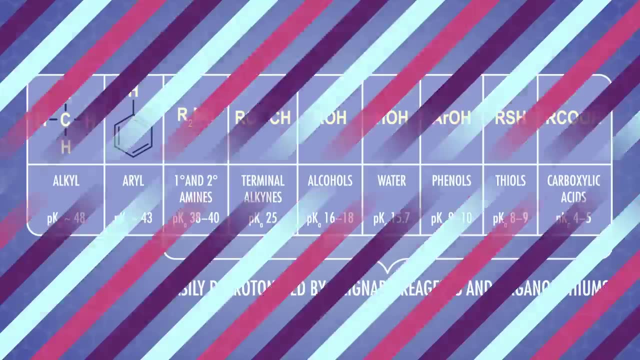 This can be a problem and we do need to watch out for acidic functional groups which could react with our Grignard in an acid-base reaction. But this basicity can also be very useful. For example, the organolithium compound n-butyllithium is basic enough to deprotonate alkynes. 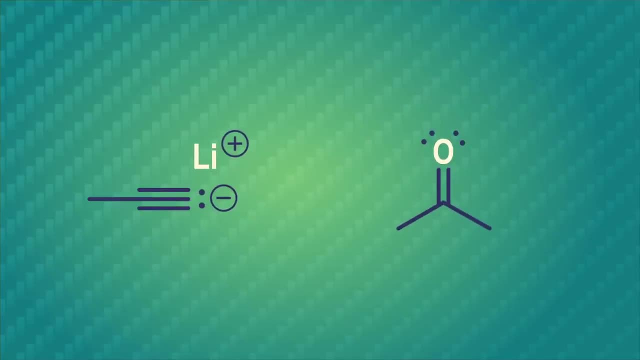 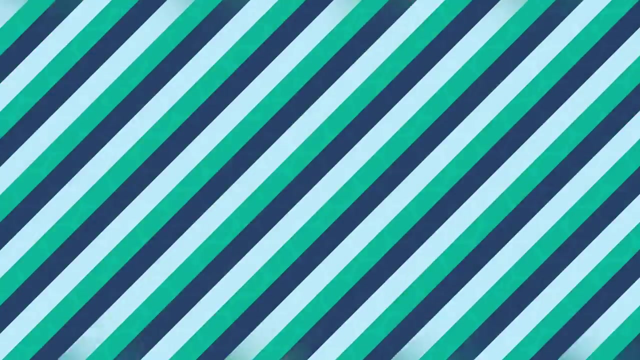 and generate an acetyl halide, As we saw in episode 27,. acetylides are powerful nucleophiles which can form new carbon-carbon bonds, Super useful for chemists. We also use organolithium compounds as our strong bases when making Wittig reagents. 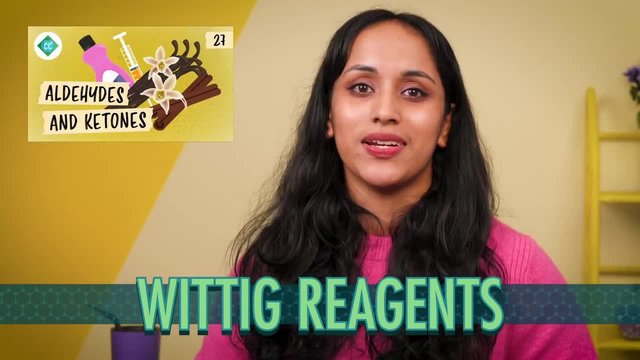 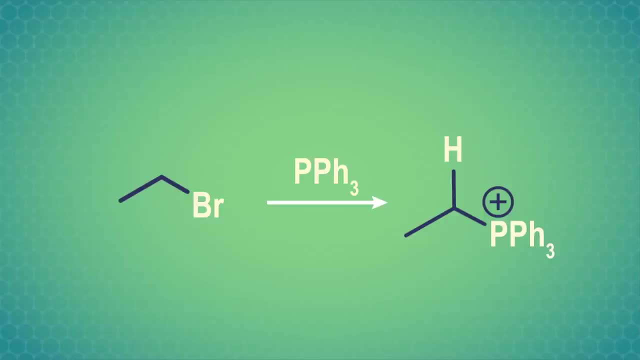 aka phosphonium illids, which we also talked about in episode 27.. First, we need to make a phosphonium salt by reacting triphenylphosphine with a haloalkane in an SN2 reaction. Head back to episode 20 and 21 for a refresher on these concepts. 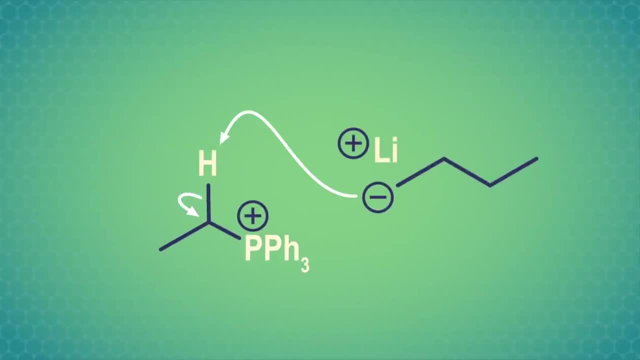 Next, we use n-butyllithium compounds, which are powerful nucleophiles which can form new carbon-carbon bonds. We also use organolithium to remove a proton from the newly formed phosphonium salt. This gives us our Wittig reagent. 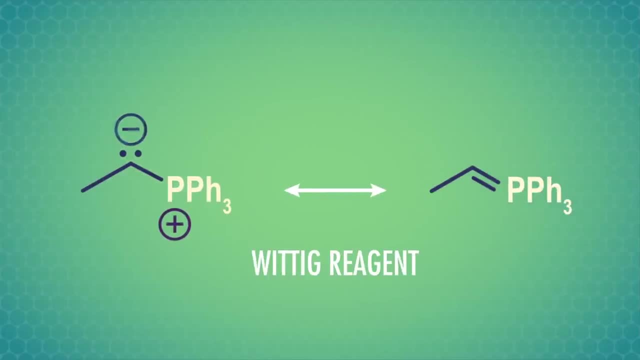 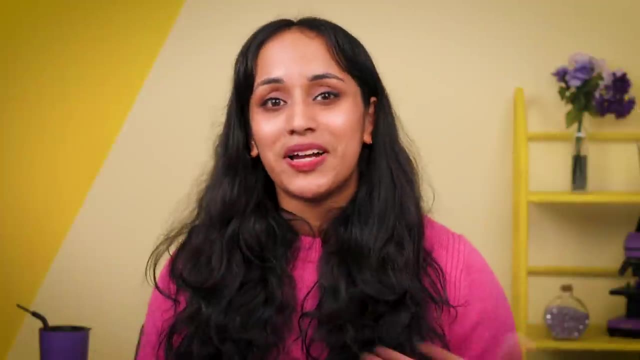 a molecule that forms a resonance structure with adjacent atoms with opposite formal charges. As a quick reminder, these can react with aldehydes and ketones to form alkenes. And since we mentioned aldehydes and ketones, we might as well get into how Grignard reagents and organolithium compounds 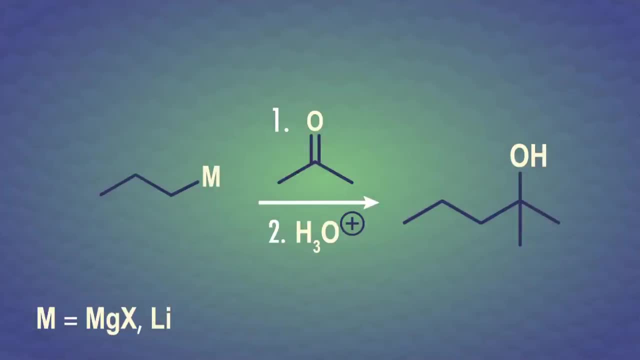 will react with these carbonyl compounds. Specifically they undergo addition reactions. The carbanion in the organometallic compound attacks the carbonyl, pushing electrons up to that electronegative oxygen. so it has three lone pairs and a negative charge. 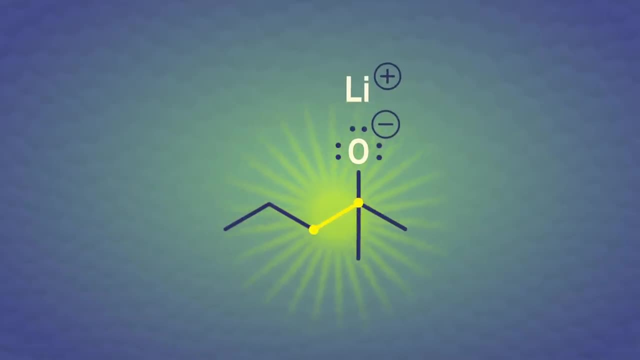 We've formed a new carbon-carbon bond, Nice. This compound will hang around until we add acid and the oxygen grabs a proton to form an alcohol And our reaction is officially done. Organometallic compounds can react with epoxides too, by opening the ring and forming an alcohol. 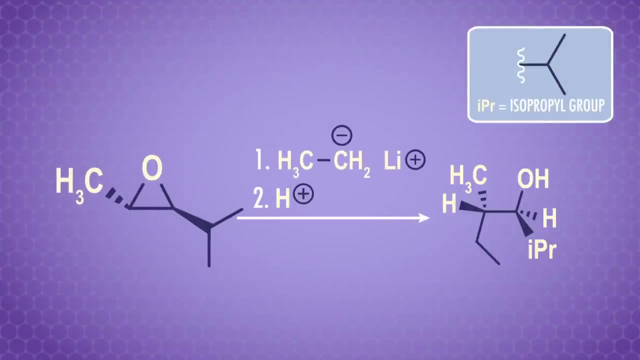 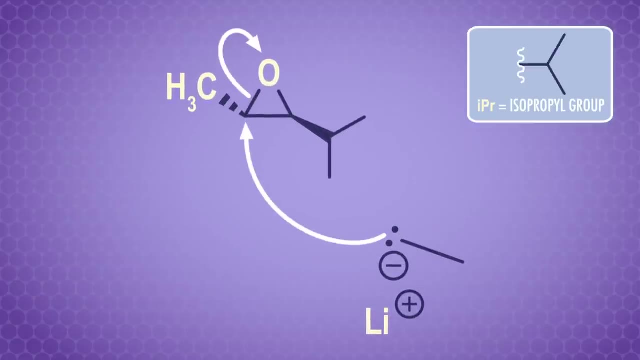 For example, let's say we have an organolithium reagent and an epoxide with two electrophilic carbons. Under these basic aprotic compounds, the carbanion does a backside attack on the epoxide, targeting the least-substituted, less-hindered carbon. 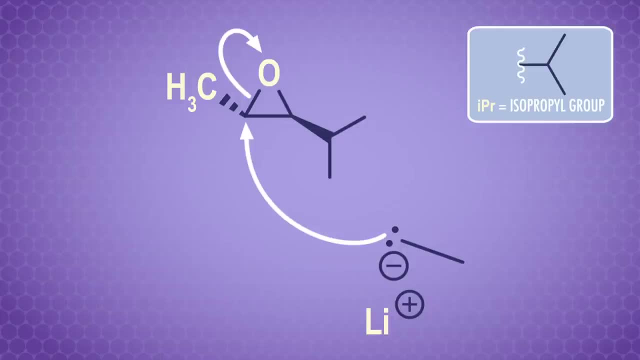 A classic SN2 reaction. We can visualize the stereochemistry of this backside attack using a Newman projection. The bonds in an epoxide are eclipsed and the oxygen atom is bridging both carbons, So the nucleophile, our organometallic reagent, carbanion. 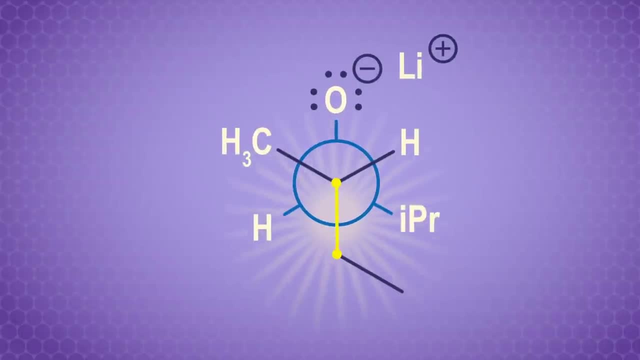 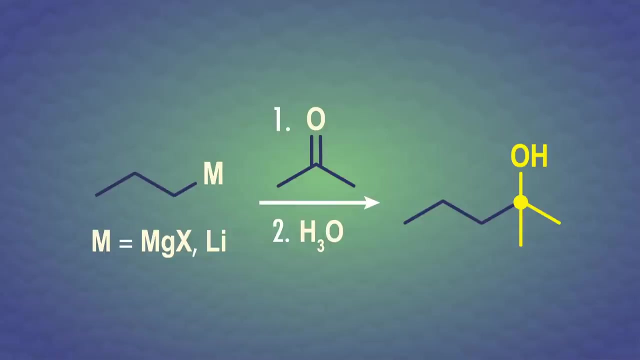 swoops in between the two groups, attacks and relieves all that ring strain. Then, like in the carbonyl addition reaction, we need some acid to form the alcohol in a second step and finish the reaction. Notice: in the carbonyl addition reaction the alcohol is directly attached to the new carbon bond. 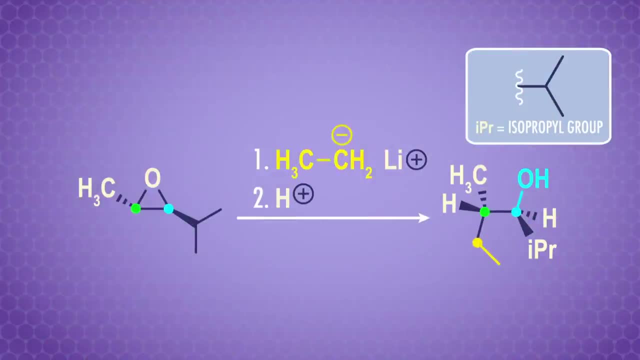 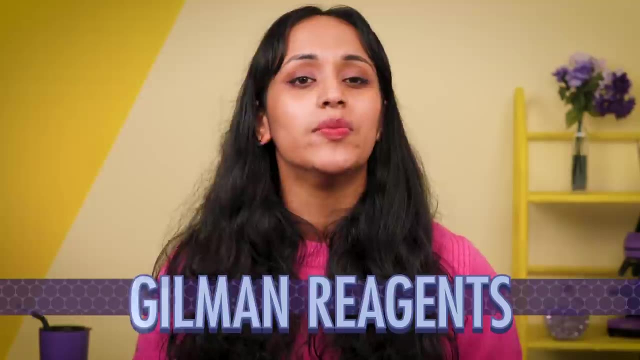 But in the epoxide SN2 reaction there's one carbon in between the alcohol and the new carbon bond. Now there's a third common group of organometallics. we haven't mentioned yet The Gilman reagents, named after the American chemist Henry Gilman. Gilman reagents contain two copper-carbon bonds and are also known as organocouperates. Now, plain old organocouper reagents which have one copper-carbon bond can't easily be made by mixing copper, metal and a haloalkane in a solvent. 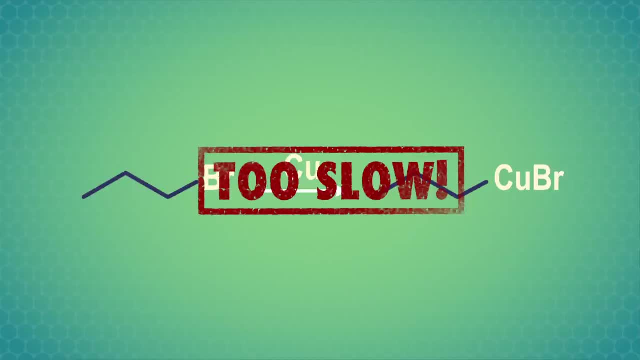 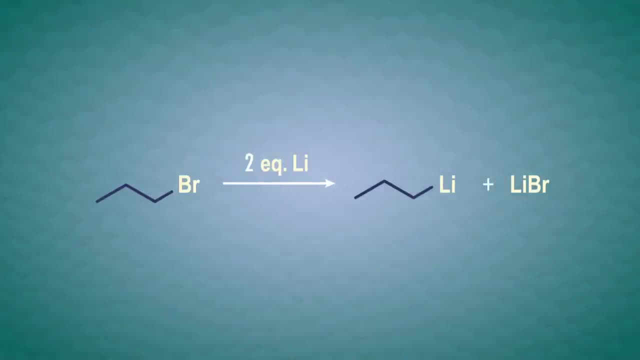 because copper is much more difficult to oxidize. Or, looking at it the other way, copper is a much weaker reducing agent than lithium and magnesium. The way around this is to start with a different organometallic, like an organolithium or a grignard. 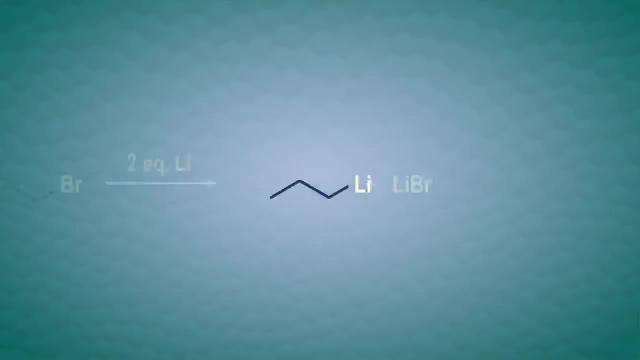 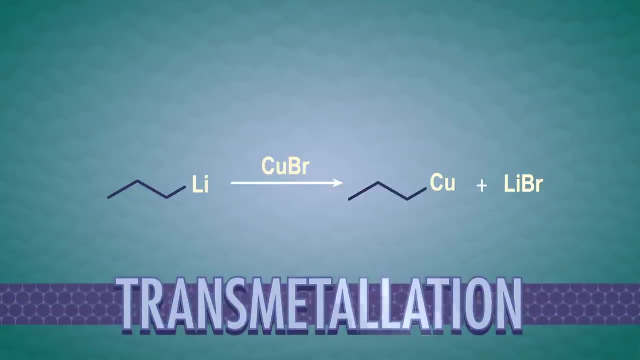 In these substances the reduction has already happened. So if we then add a copper salt, like copper bromide or copper chloride, the metals are exchanged in a process called transmetallation, which gives us our organocopper. Organocopper reagents are less reactive than the other organometallic reagents we've been talking about. 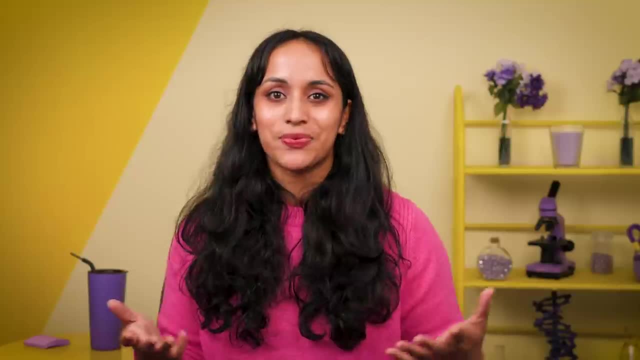 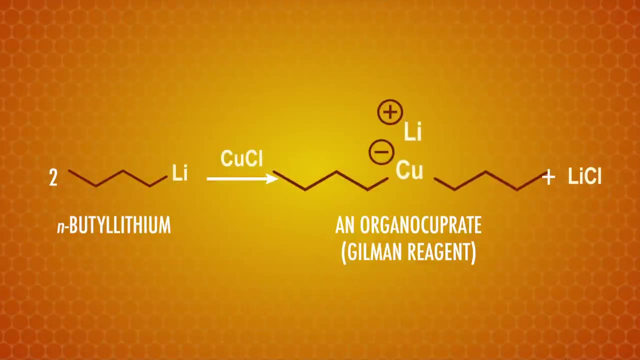 so we don't have to worry quite as much about intense reactions with air that will catch our lab bench on fire. But they can also be too unreactive to be very useful. That's where Gilman reagents with two carbon-copper bonds come in. 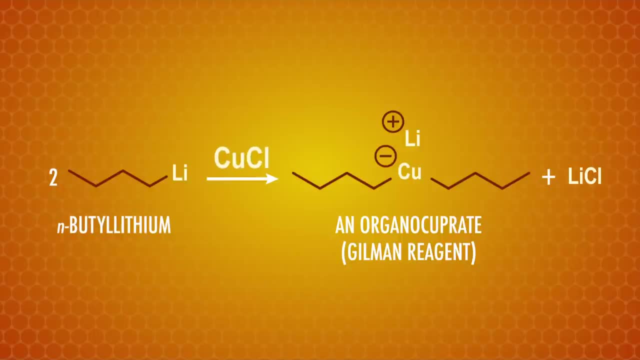 To form an organocouperate. we add a copper-1 halide to two molar equivalents of an organolithium. The name has an A in it. It's called a halide. It has an 8,, which suggests a negative ion. 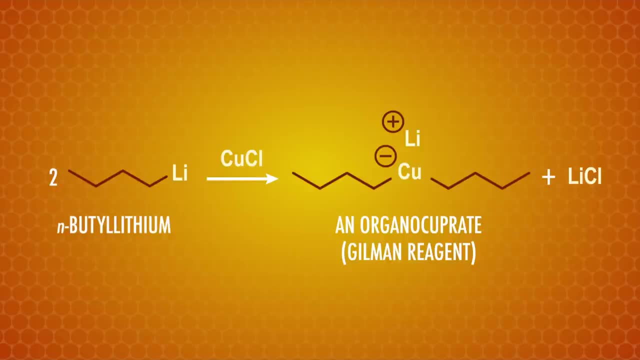 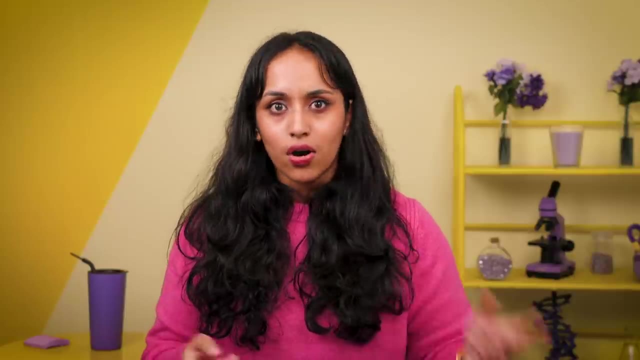 Think sulfate carbonate nitrate. This 8 tells us that organocouperate reagents have a negative charge. Even though organocouperates are more reactive than organocoppers, they aren't as reactive as grignards and organolithiums. 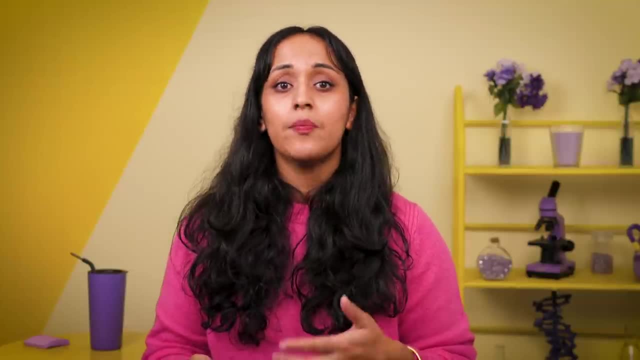 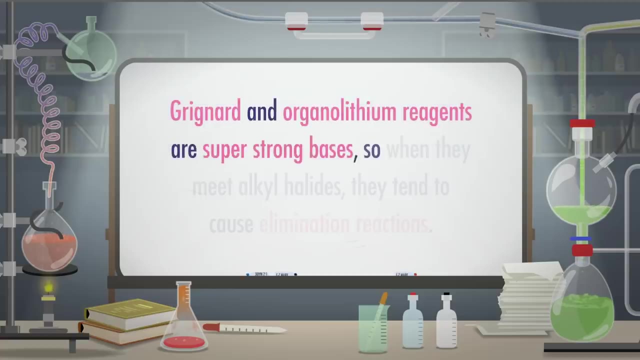 But Gilman reagents have an advantage in their not-so-basicness because they can get involved in other types of reactions. Grignard and organolithium reagents are super strong bases so when they meet alkyl halides they tend to cause elimination reactions. 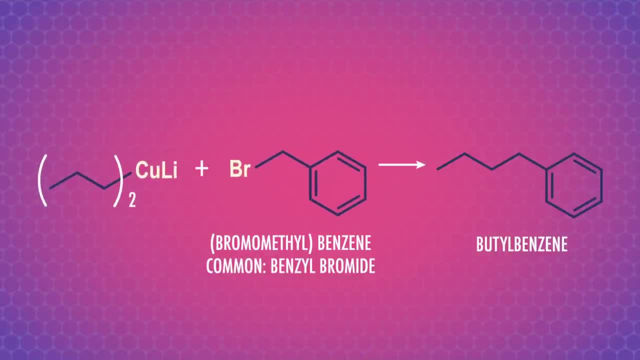 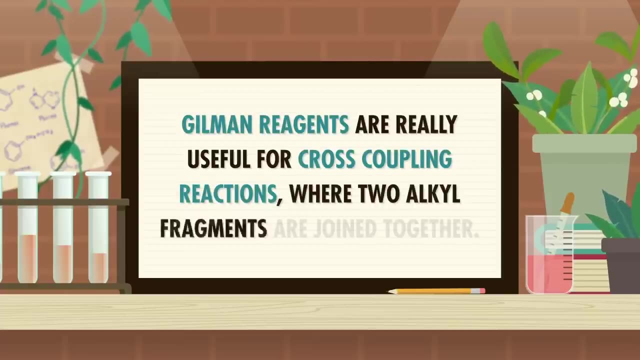 However, when Gilman reagents meet alkyl halides, they do SN2 reactions instead. In fact, Gilman reagents are really useful for cross-coupling reactions, where two alkyl fragments are joined together. The mechanism is a bit beyond the scope of the series. 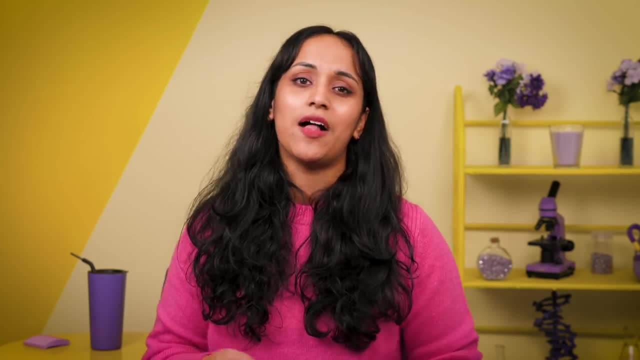 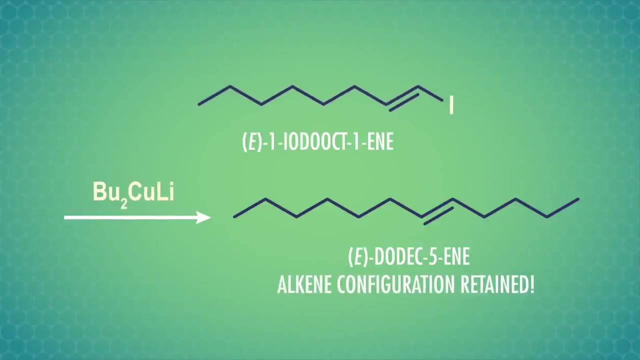 but basically one of the alkyl bits in the Gilman reagent joins up with the alkyl bit of the alkyl halide. Gilman reagents can also undergo cross-coupling reactions with haloalkenes, while preserving the stereochemistry of the double bond. 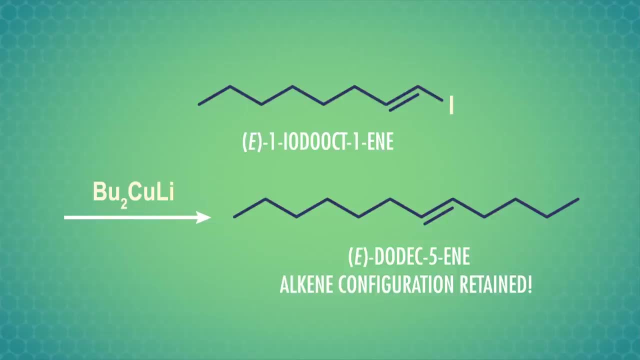 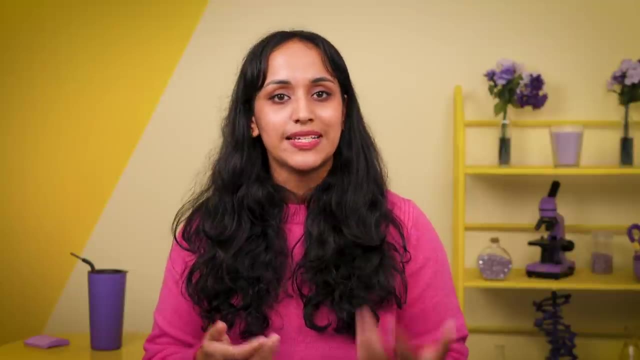 Since we can't do SN1 or SN2 reactions with these vinyl halides, this is a pretty handy new reaction. Also, the carbon-copper bonds in Gilman reagents are less polarized than carbon-magnesium or carbon-lithium bonds. 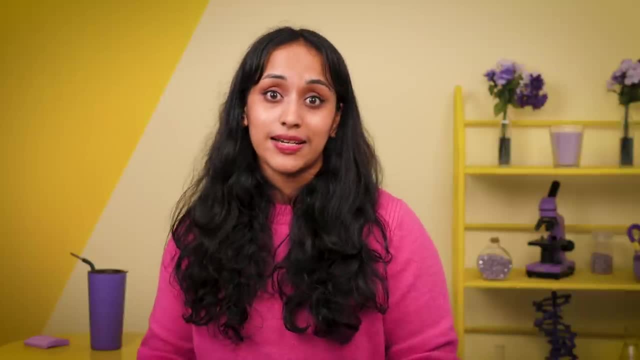 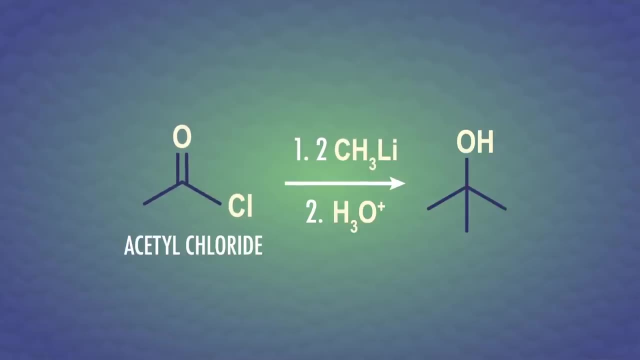 This makes Gilman reagents less reactive and therefore more selective. For example, if we mixed a grignard or an organolithium with an acetyl chloride, two molecules of the reactant would add to the carbonyl carbon, eventually forming an alcohol. 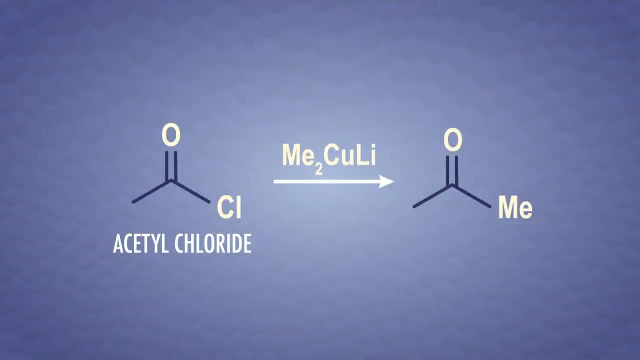 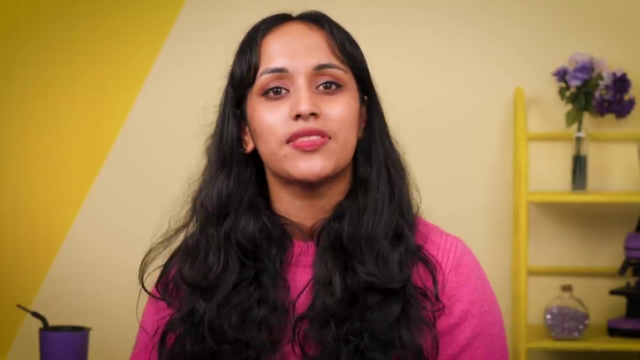 However, if we mixed a Gilman with the acetyl chloride, the chloride swaps with the acetyl halide, leaving the carbonyl in the final product. So, while learning about all these organometallics, we've talked about the toxicity of tetraethyl lead and the reactivity of grignard reagents. 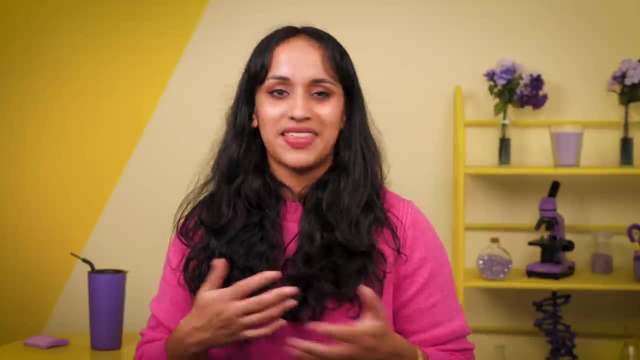 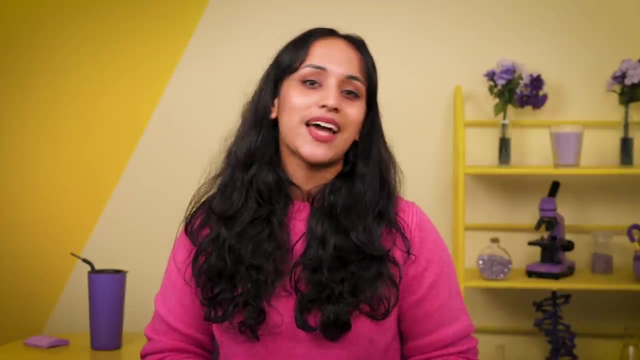 But more stories are out there. For example, in one of his Things- I Won't Work With articles- the medicinal chemist Derek Lowe relates the story of the Library of Congress in the US trying to use diethyl zinc to deacidify old documents in the 1980s and 90s.